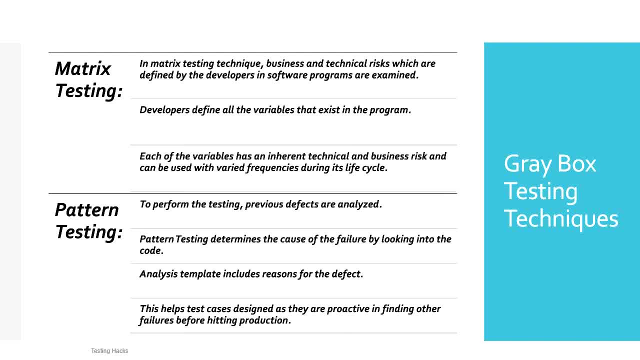 where it is: matrix testing, pattern testing, orthogonal testing and regression testing. okay, the first one is matrix testing. in matrix testing technique, business and technical risks, which are defined by the developers in software programs, are examined. developers define all the variables that exist in the program. each of the variable has an inherent technical and business risk and can be. 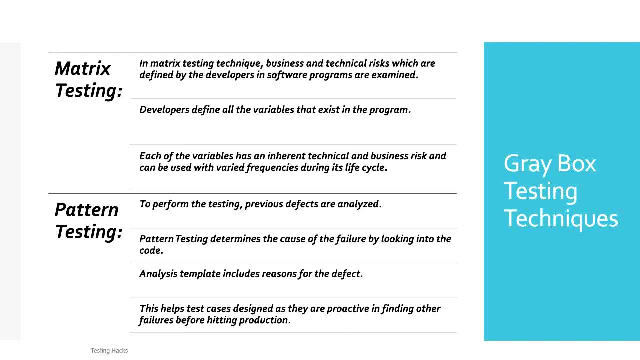 used it with varied frequencies during its lifecycle. when it comes to pattern testing, it is used to perform the testing. previous defects are analyzed. to perform the testing whereon the previous defects are analyzed. pattern testing determines the cause of failure by looking into the code analysis template. includes reason. 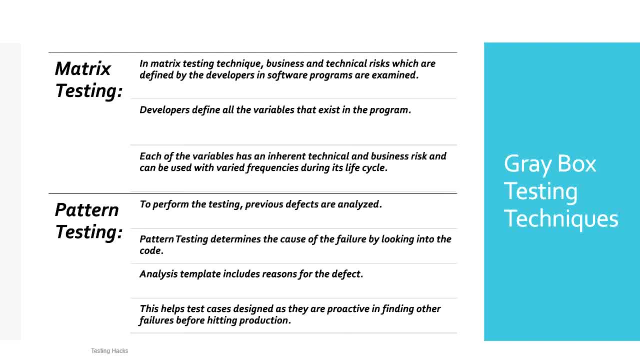 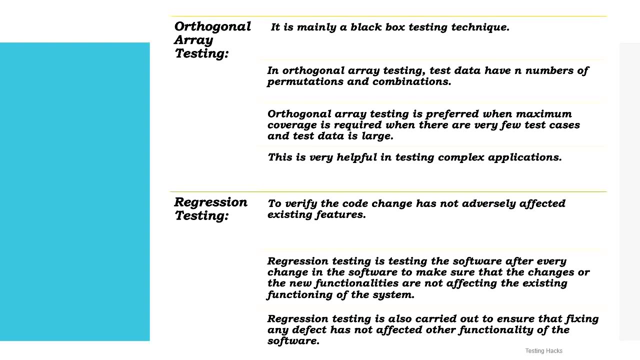 for the defect. this helps best cases design as they are proactive in finding her, finding other failure before hitting production. next technique is orthogonal array testing. it is mainly a black box testing technique. in orthogonal array testing test data have n number of permutation and combinations. orthogonal array testing is preferred when maximum coverage is required when 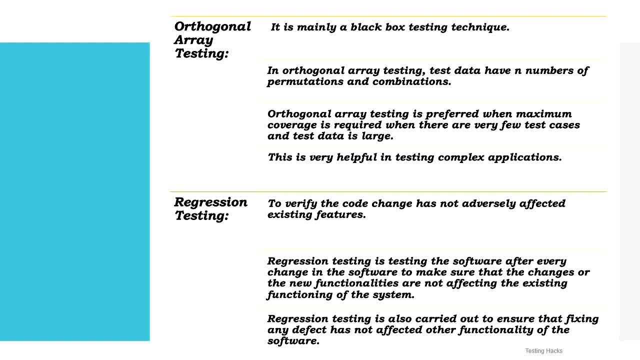 there are very few test cases and test data is large. this is very helpful in testing complex applications. and coming to regression testing, to verify code change has not adversely affected the existing features, we will perform the regression testing. regression testing is a testing the software after every change in the software to make sure that the changes or the new functionality. 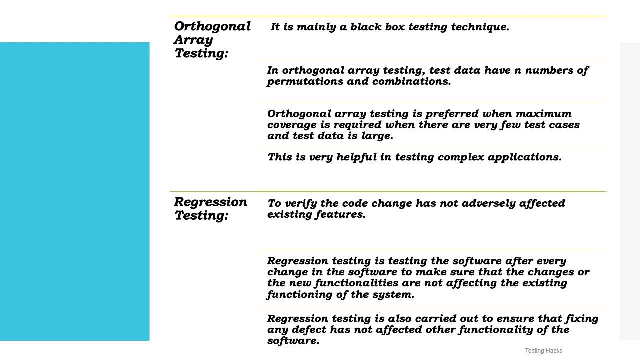 are not affecting the existing functionality of the system. regression testing is also carried out to ensure that the fixing any defect has not affected other functionality of the software. so these are the four different techniques we have in gray box testing. so we will look at an example how we can. 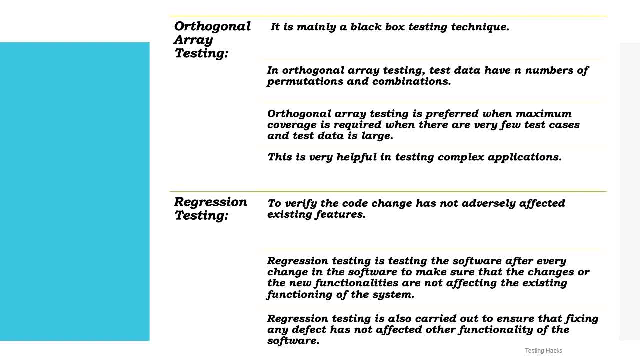 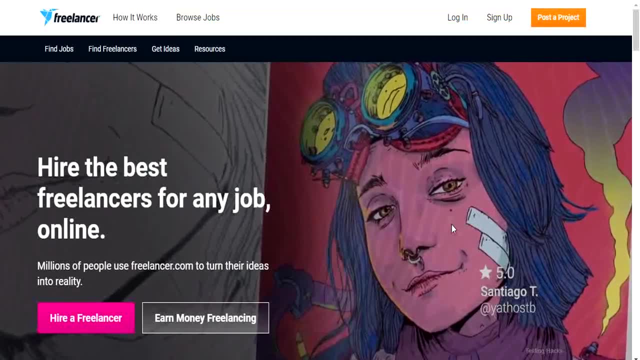 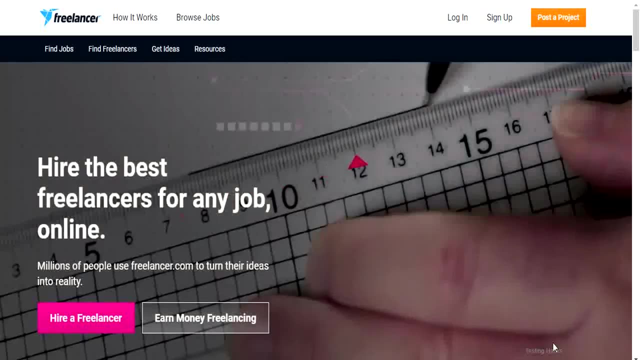 perform gray box testing even with having little code knowledge as well as not knowing much code knowledge in between, which is a partial kind of testing. ok, we will do that now. here I have taken an example of freelancing homepage. ok, so on this main website we will try to do some changes. 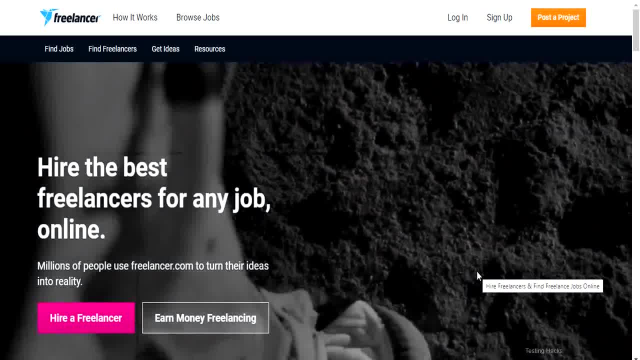 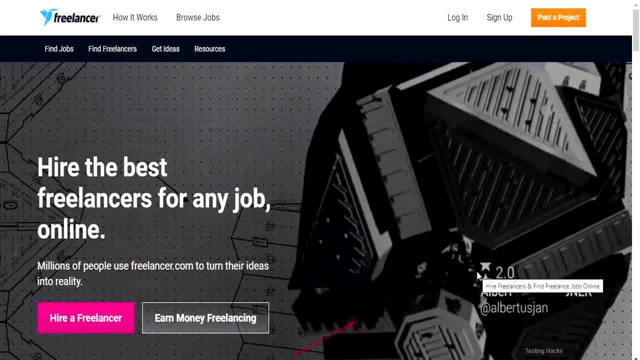 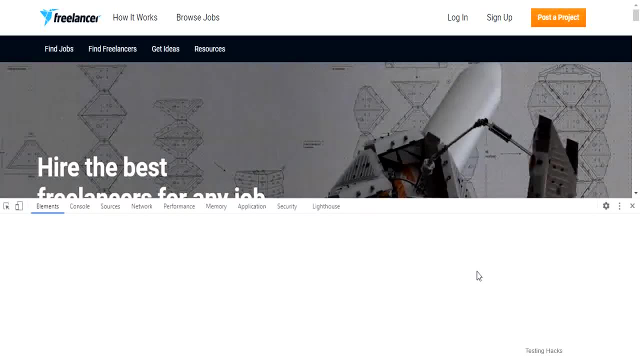 using the browser itself. so once you are in this page, we have developer tools. you might be knowing developer tool. if you don't know, just hit on f12. okay, you will get the developer tool window like this, okay, so where you can see that, all the elements here, which is the 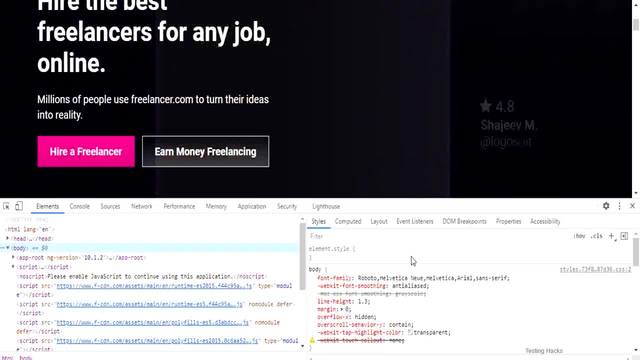 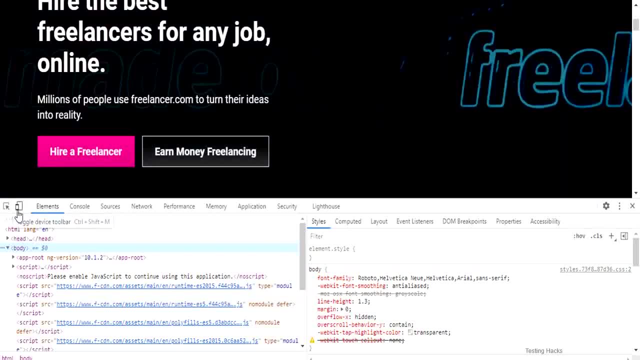 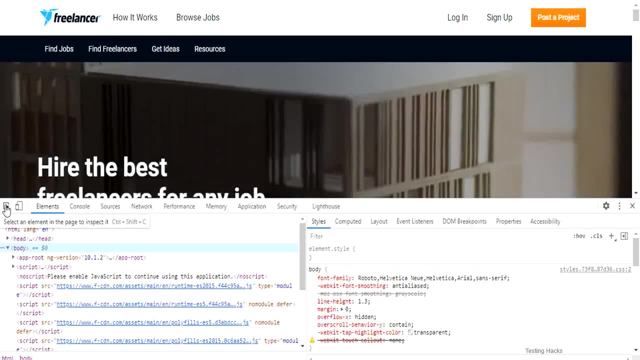 html element. you can find it here- and these are the css styles where the styling of the application has been done. okay, so let's try to do some kind of- uh, you know- freshening activity here. so click on this arrow- kind of thing you are able to see right, so hit on this. so let's do some. 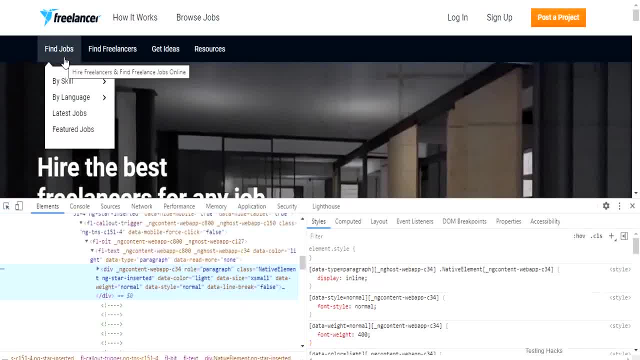 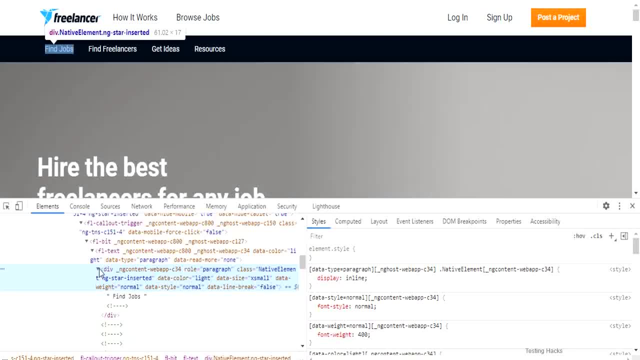 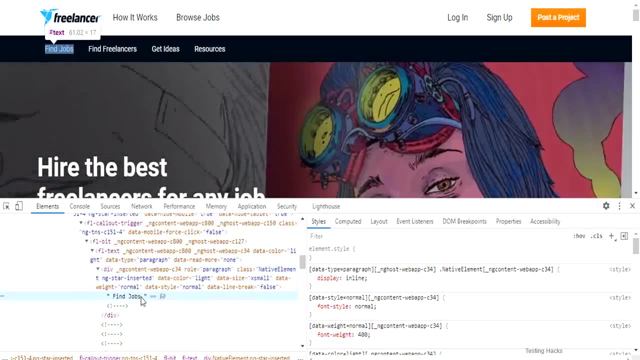 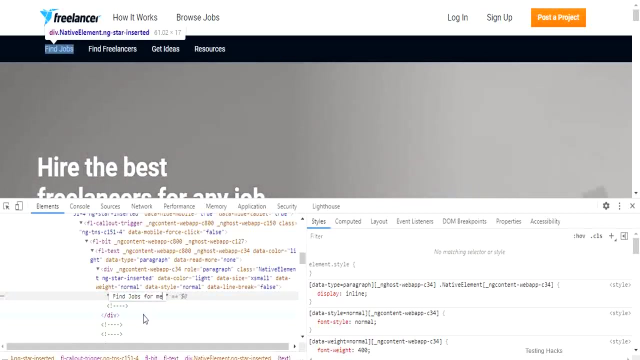 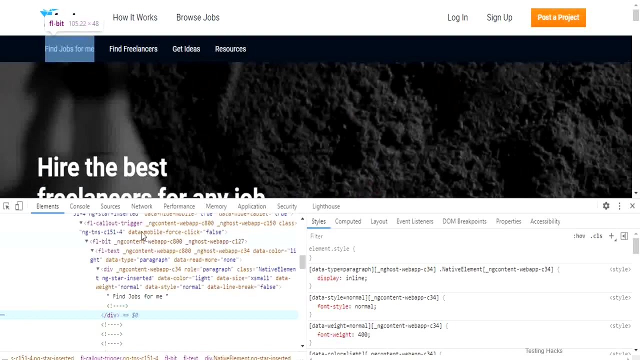 changes on the header. okay, so i clicked on this. okay, so, which will highlight the particular element uh in the uh, you know, html, html. so i want to change this to find jobs for me. so what i'll do? i'll just click on this: find jobs for me. okay, see, did you see that it updated my text, suppose, say, in real time. 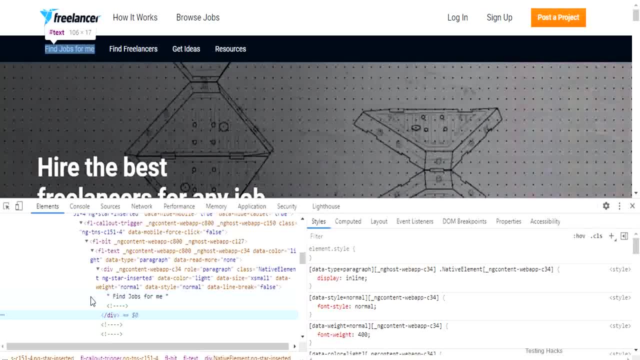 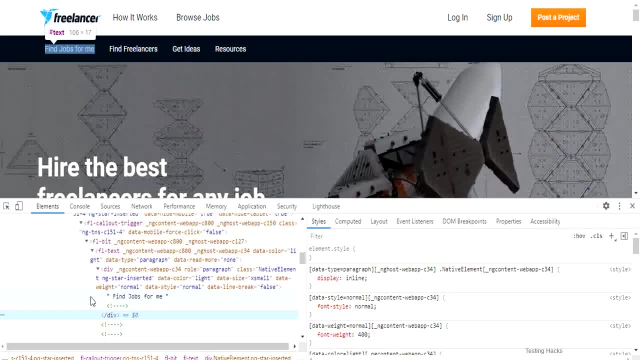 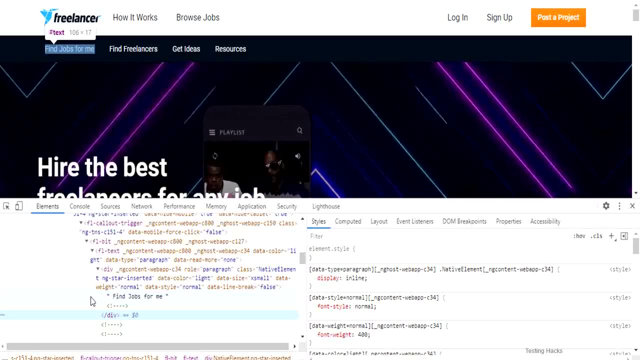 what happens. you are facing some ui kind of issues that you can actually debug by yourself, rather than going to developer tool developer so that you can tell the developer that you can do these changes, but these are only for your browser, you are not deploying it or you are not doing the changes in the real time. it is only 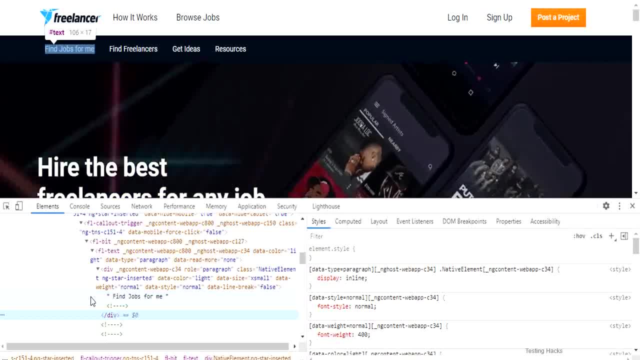 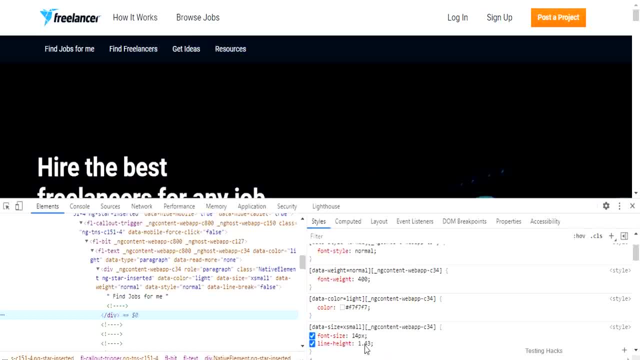 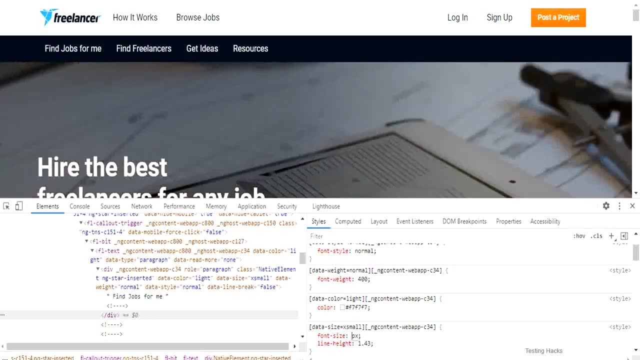 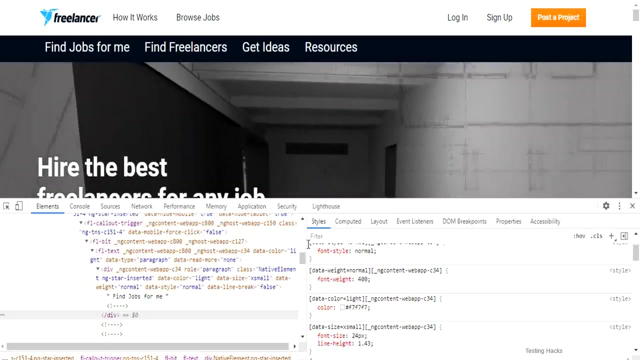 for your browser. you are trying to do some changes, okay, so what else we will do is here we can see some css style, right? uh, let's change the font of all the header, you know, navigation, uh, menu, to something like 20, something like 24. okay, it was 14 before, so i updated it. did you see that? it got updated, okay.